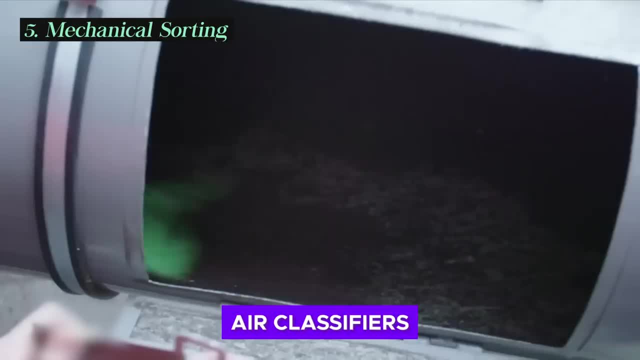 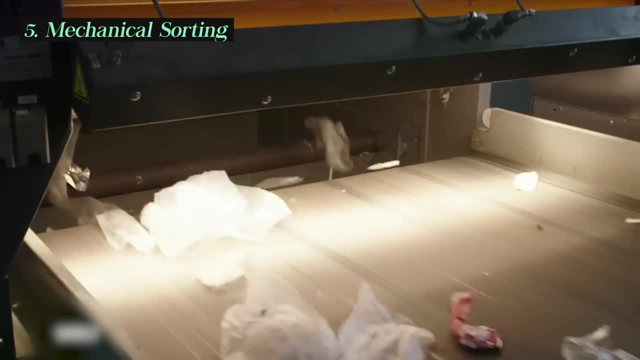 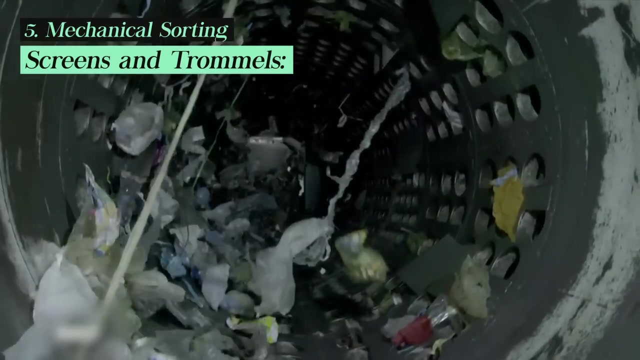 Finally, automated conveyor belts. screens, air classifiers, magnets and optical sensors are some of the equipment used to sort materials based on their properties, such as size, weight, shape and material type. These rotating cylindrical screens separate materials based on size—smaller items fall through, while larger items continue down the conveyor. 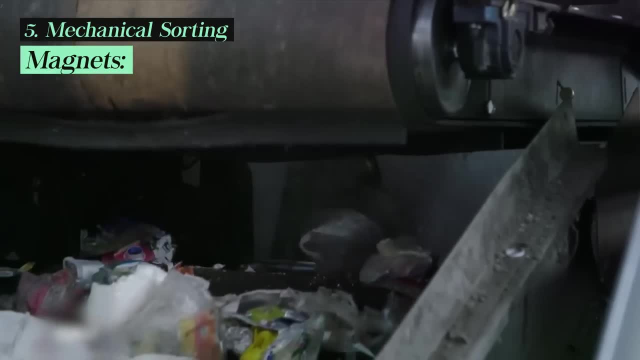 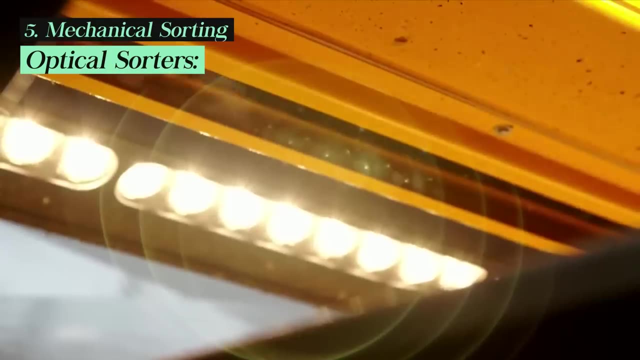 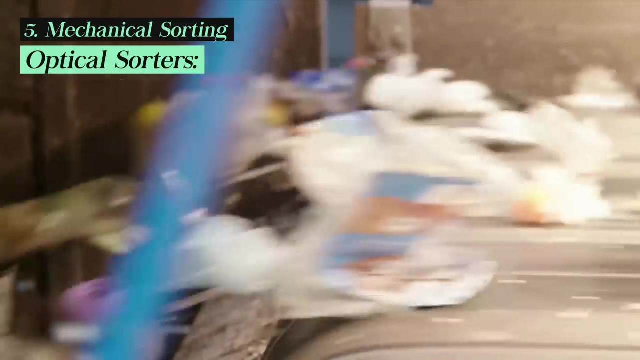 Powerful magnets are used to attract and separate ferrous metals containing iron, such as steel cans ently sensors and cameras to identify and separate materials based on their optical properties, such as color and shape. they can sort plastics by resin type and colors. air jets are used to separate lightweight materials like 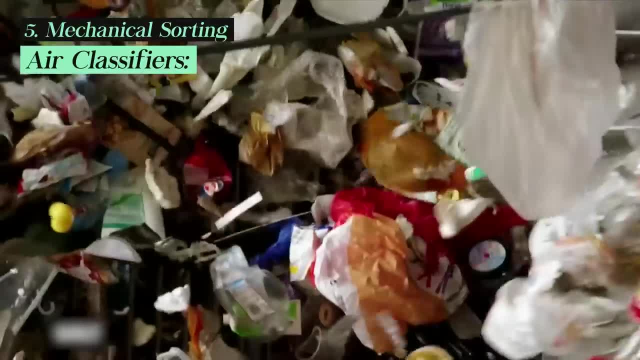 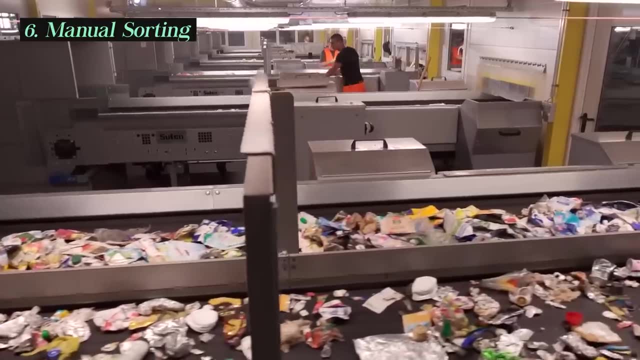 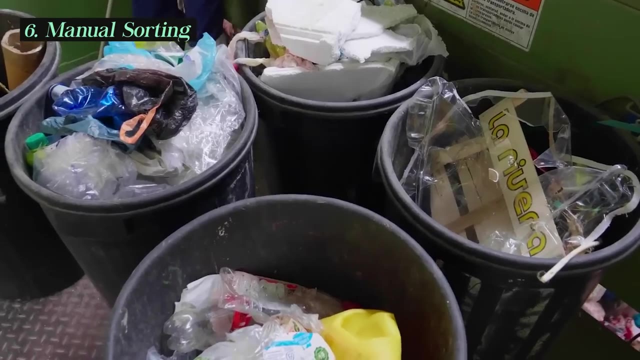 paper and plastic from heavier materials like glass and metal. despite advanced technology, manual labor remains important in the sorting process. workers stationed along the conveyor belts manually remove contaminants as well as items that the automated systems may have missed. manual sorting helps ensure higher quality recyclables. after sorting, the separated materials are compacted or 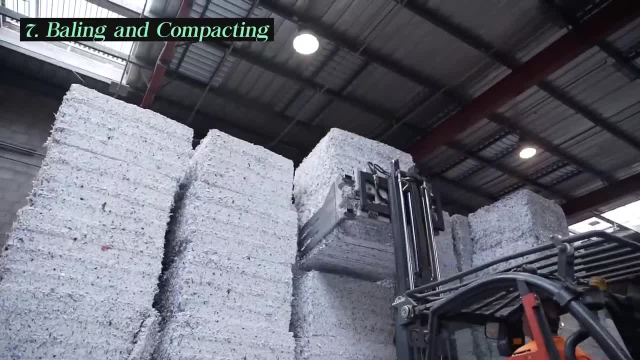 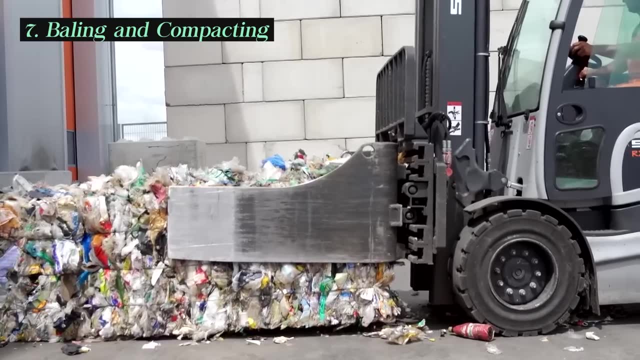 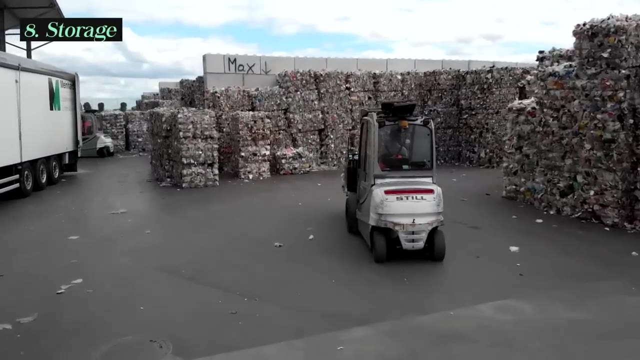 bailed bailing involves compressing materials like paper, plastic, cardboard and aluminum into large blocks or bales. this process makes the materials easier to handle, store and transport. bales of sorted recyclables are stored in the MRF until they're ready to be transported to manufacturers for further 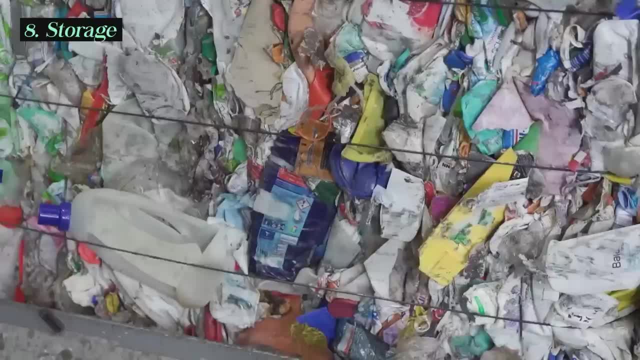 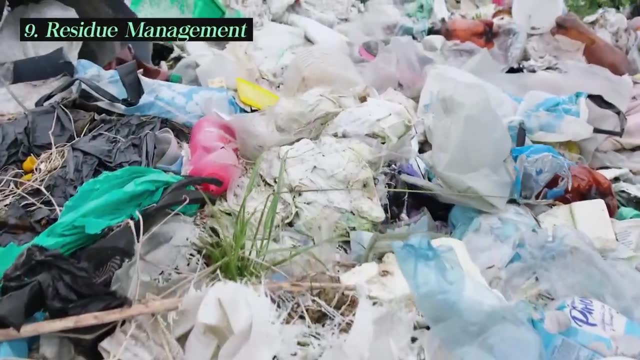 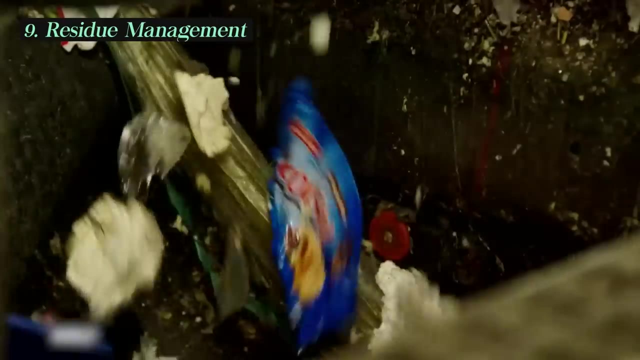 processing. proper storage helps ensure that the quality of recyclable materials is maintained. some non recyclable or difficult to recycle items, known as residue, may still be present in the sorted materials. MRFs manage this residue, which may include items like plastic bags, food waste and small non. 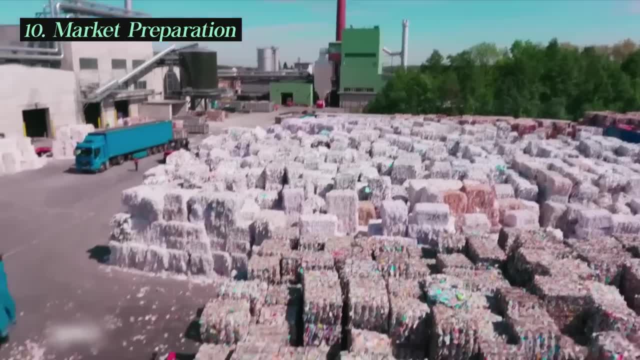 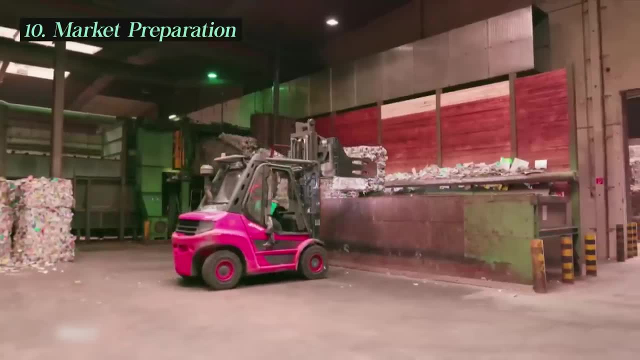 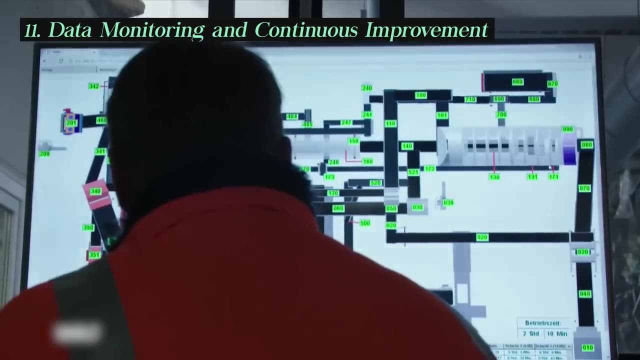 recyclable pieces. once bailed and sorted, the recyclables are sold to manufacturers and processing facilities as raw materials. these materials will be used used to produce new products, reducing the need for virgin resources. Many modern MRFs use data tracking and monitoring systems to measure efficiency. track contamination. 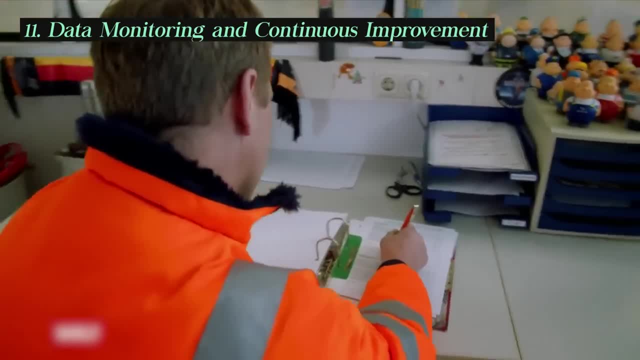 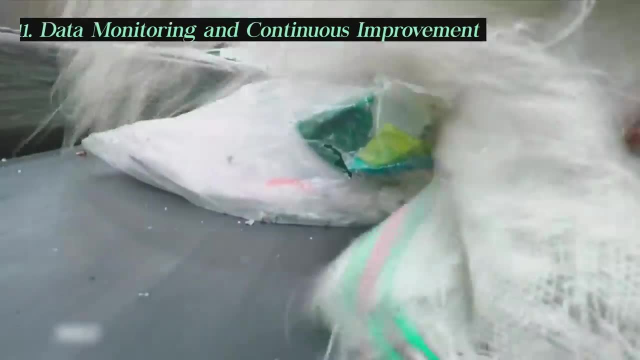 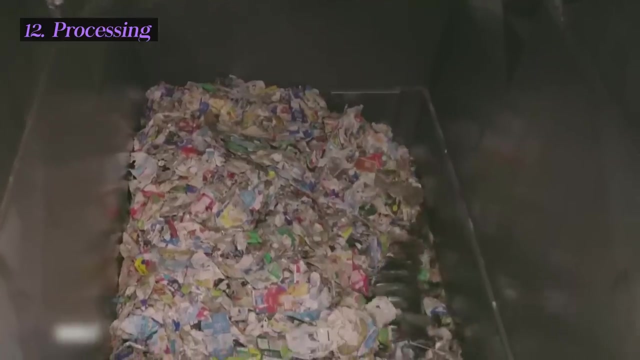 rates and identify areas for improvement in the sorting and processing processes. This data-driven approach helps optimize operations and enhance recycling outcomes. Once sorted by the MRF, the materials are then transported to processing plants, where they're subjected to specific processing methods based on their types. 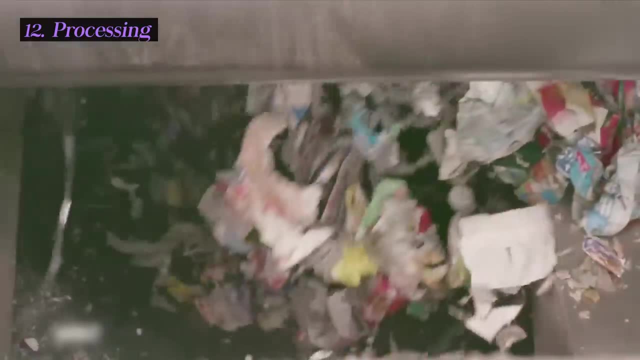 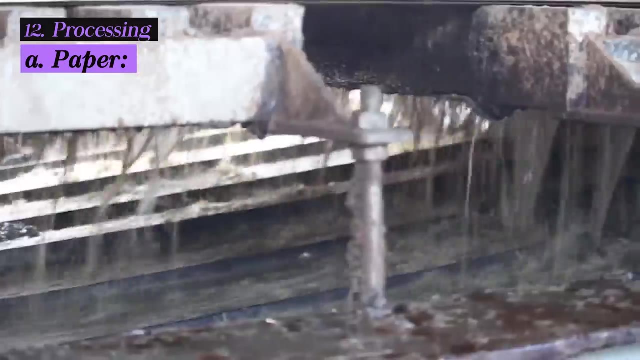 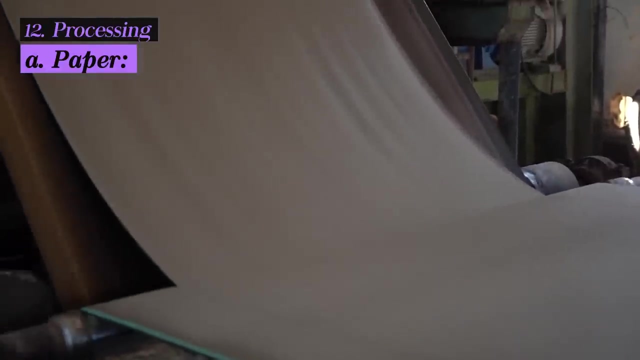 Each material type requires unique treatment to prepare it for reuse. A Paper Paper is often shredded and mixed with water to create a pulp. This pulp is then cleaned and refined, removing ink, adhesives and other impurities. The resulting pulp can be used to produce new paper products. 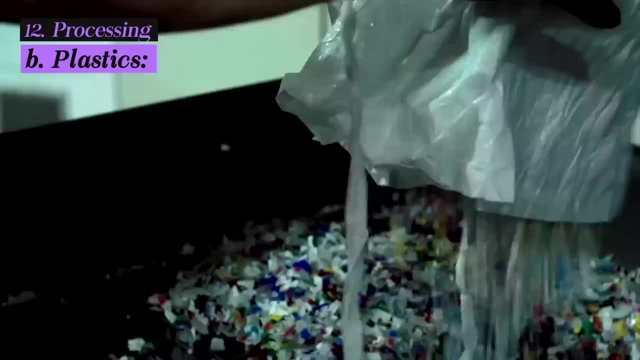 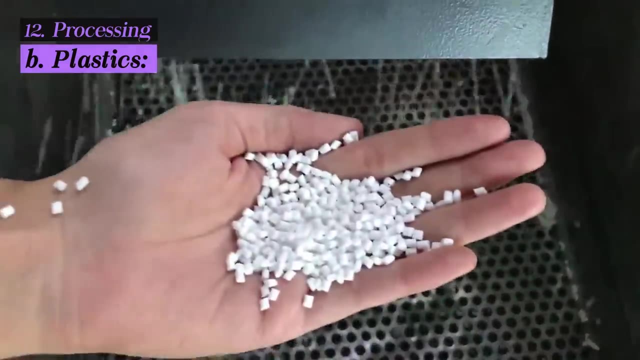 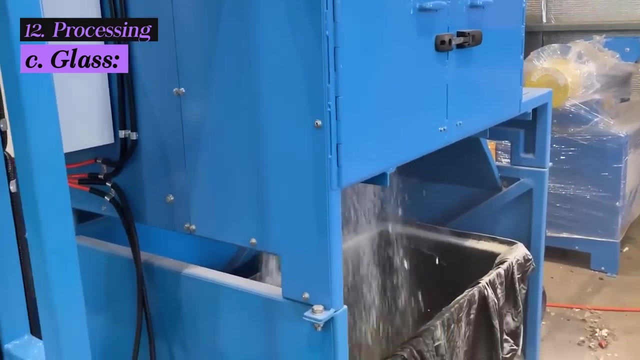 B Plastics. Plastics are sorted by type and then undergo processes such as shredding, washing and melting. Plastic pellets serve as the raw material for manufacturing new plastic products. C Glass: Glass is crushed into small pieces, known as cullet. 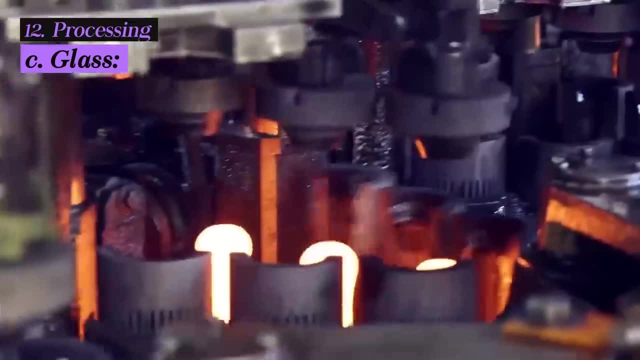 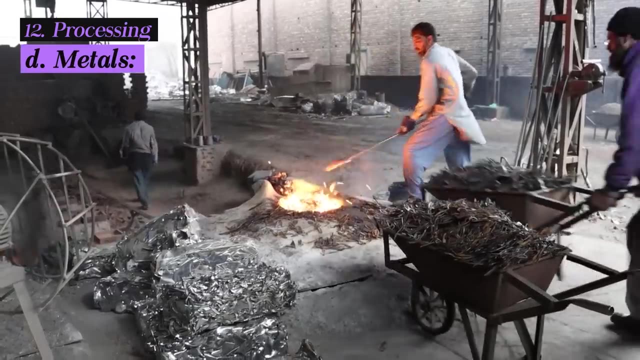 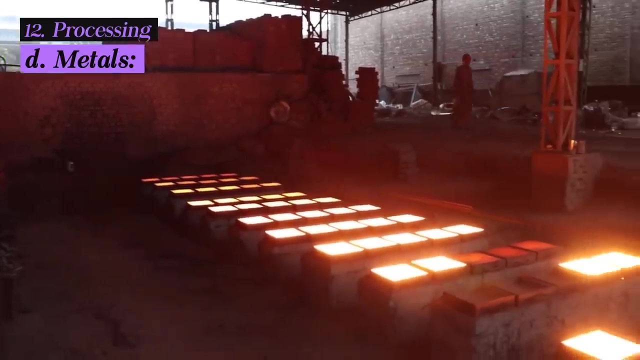 The cullet is melted down to produce new glass products, reducing the need for raw materials and energy compared to making glass from scratch. D Metals- Metals like aluminum and steel- are melted down to form ingots or sheets. The recycled metal can be used to manufacture plastic. 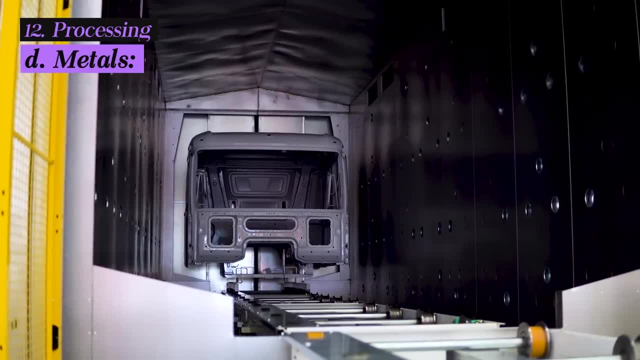 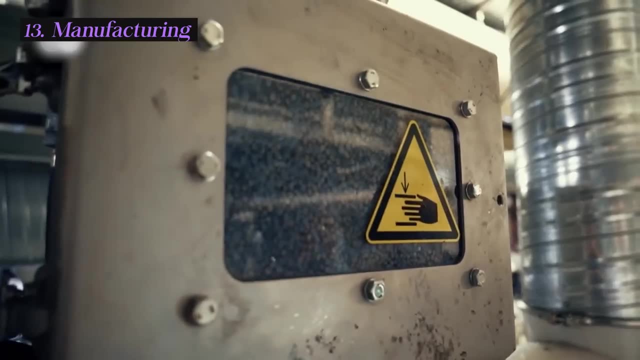 The recycled metal can be used to manufacture a wide range of products, from cans to car parts. Processed materials are sent to manufacturers, who use them as inputs for creating new products. The use of recycled materials in manufacturing reduces the demand for virgin resources, conserving. 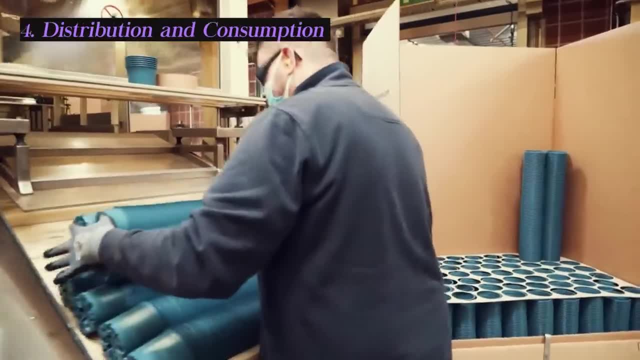 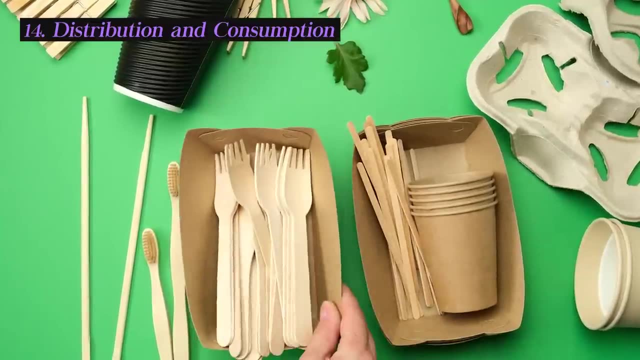 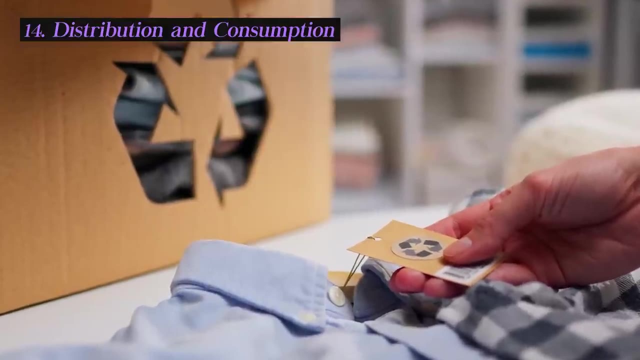 energy and reducing greenhouse gas emissions. The newly manufactured products are distributed to consumers through retail outlets. These products made from recycled materials offer the same quality and functionality as those made from recycled materials. By purchasing and using these products, consumers support the closed-loop recycling system and 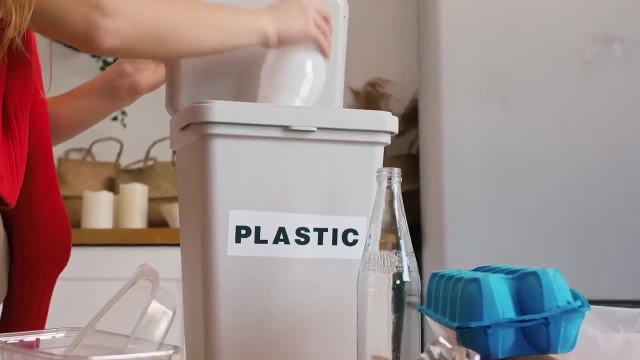 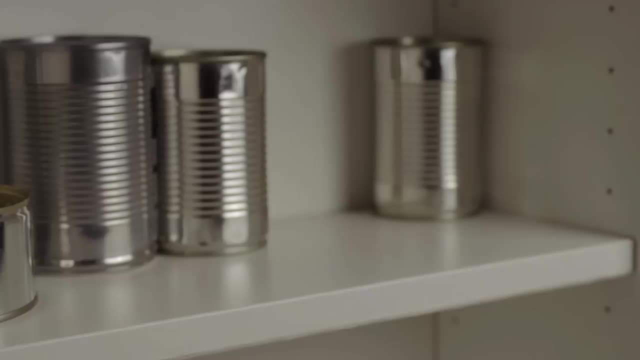 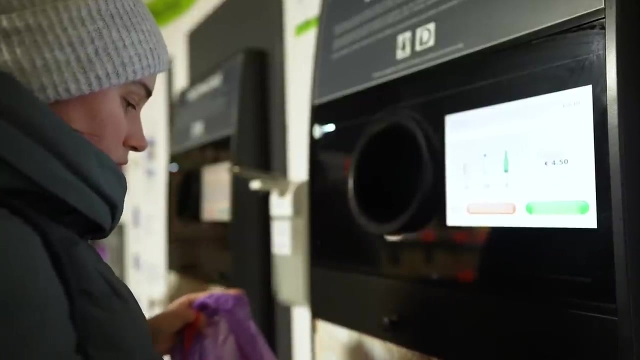 promote sustainable practices. Eventually, recycled products may reach the end of their useful life. At this point, some materials can be recycled again, continuing the cycle. For instance, aluminum can be recycled indefinitely without losing quality. Other materials might have limitations on the number of times they can be recycled due 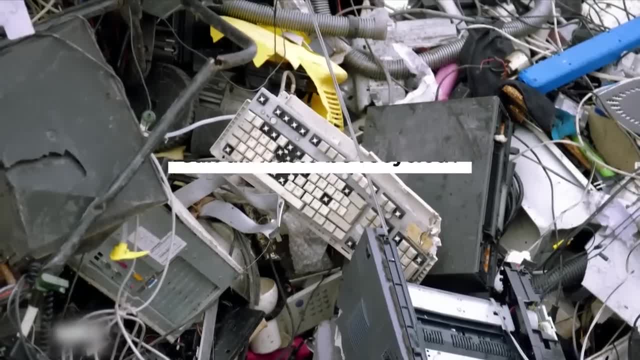 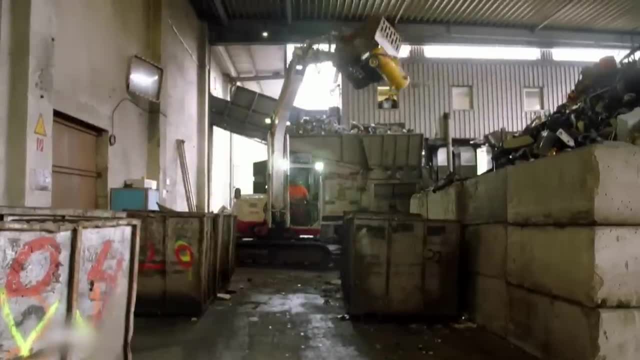 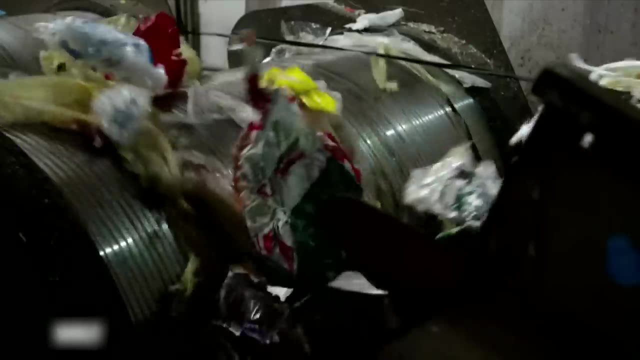 to degradation. Let's return to our topic: Can all waste be recycled? If not, how much of it isn't recycled? Well, the answer is: not all waste can be recycled, due to technical, economic or environmental constraints. As far as percentages go, 60% of the waste that ends up in a recyclable can is not recyclable.